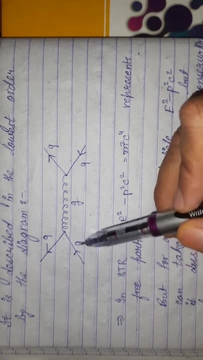 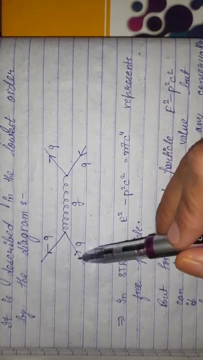 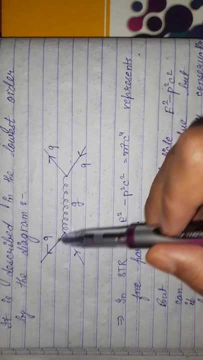 form a baryon. a baryon is made up of quark and anti-quark. so we have a quark and we have an anti-quark and which is, uh, which is actually bounded by the help of gluons, which is the carrier of force in here and simply in that we have seen in in case of the Feynman diagram of qed. 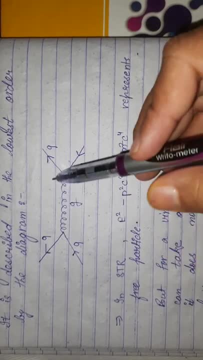 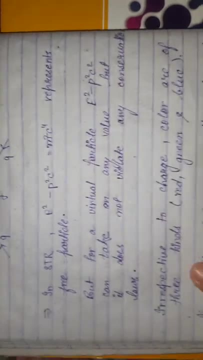 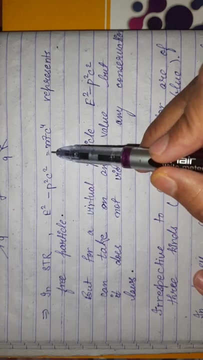 where q was replaced by e electron and g was replaced by photon. it is just a simple representation. it is as same as that was now in hdr. we represent in a special theory of relativity. we represent e square minus p square. c square is equal to m square c to the power 4. this actually represents. 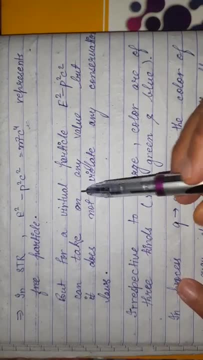 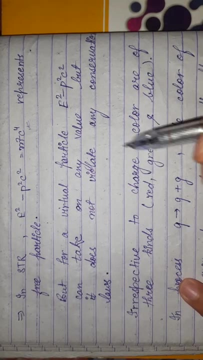 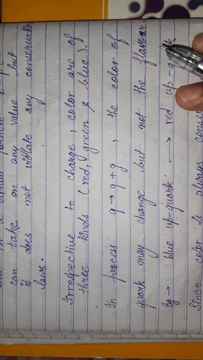 a free particle. but in case of virtual particle, e square minus p square, c square can take any value. okay, it can take any value just to satisfy conservation law, but it cannot violate any conservation law. okay, irrespective to charge. color are the three? are of three kinds, i mean. 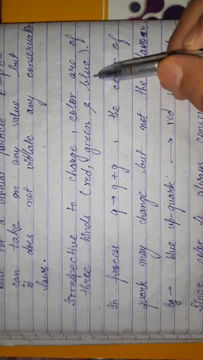 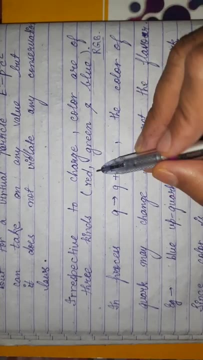 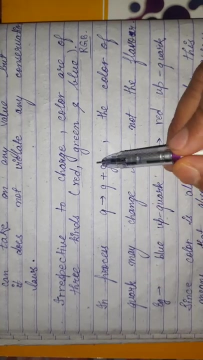 color. we we have color of three kinds: red, green and blue rgb. you can call it as rgb. similarly, we have anti-color, that is, anti-red, anti-green and anti-blue. okay, in process, q tends to q plus g- g is actually gluon and q square copy as representation. and 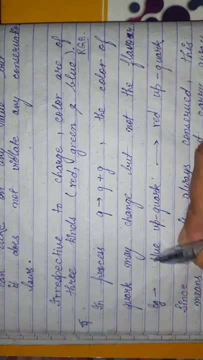 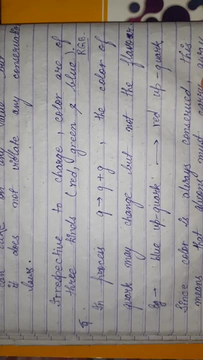 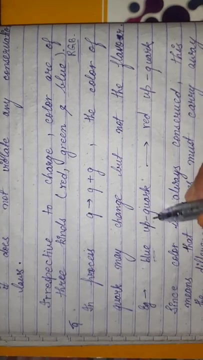 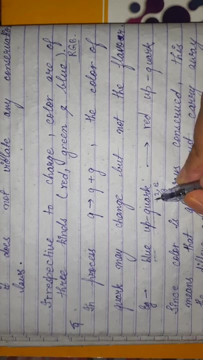 q is represented as anti-quark. ok, the colour of quark may change, but not the flavour. now, what is the flavour and colour we will see here? that suppose there is a quark with blue, but it is up quark, and we know up quark contains two by three times of charge, okay, plus TWO BASE Wheel times of. 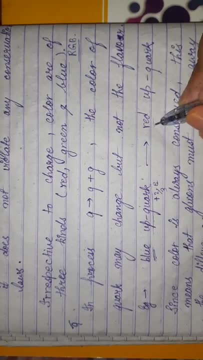 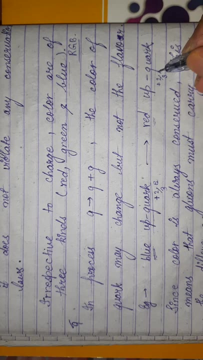 than what we later have to do to figure out it where there's a challenge. but now the color has changed into red and the quark remains the same. i mean, quark's value of charge remains the same. that means the flavor of quark has not changed. that is the charge. 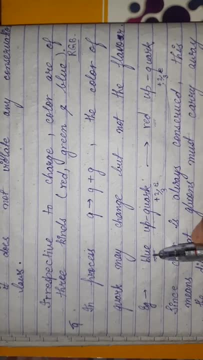 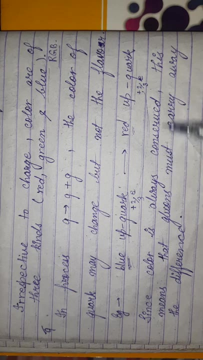 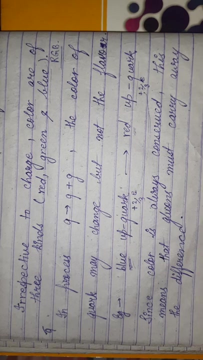 that quark had earlier is not changed, but only the color has changed. okay, it has converted from blue to red. now, since color is always conserved, this means that gluons must carry away the difference, like charge is always conserved. we have here that color must always be conserved. 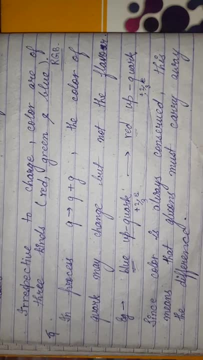 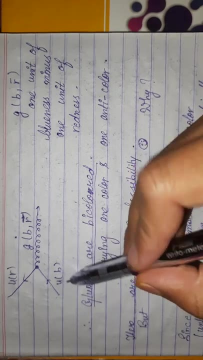 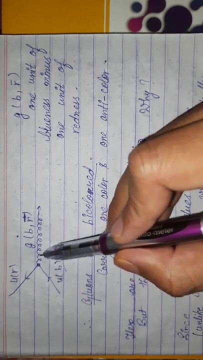 that means that there must be something that has to balance these things, and that is gluon. okay, so in here we can see that up quark with blue color has changed into up quark of red color. now the carrier that is known as gluon has is made up of two colors: one is blue, one is blue and the 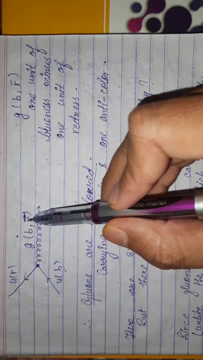 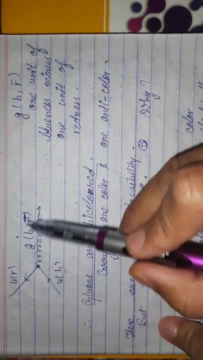 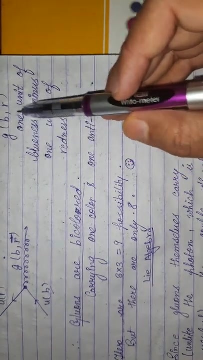 other one is r bar. r bar is actually anti-red color, anti-red color, so that anti-red color and red color mixes up and gives white color and we- only we are only left with blue color. okay, here how to represent it. g of b comma. r. r bar. one unit of 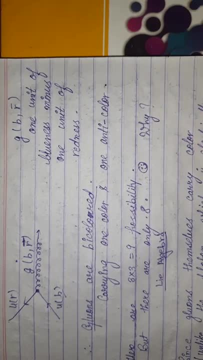 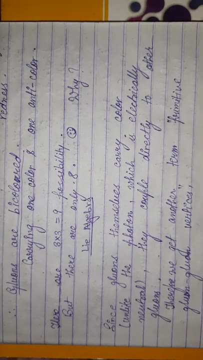 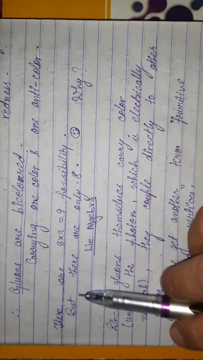 blueness minus one unit of redness. okay, now gluons are bicolored. gluons always have two colors. okay, carrying one color and one anti-color. there are three cross three is equals to nine possibility, but there are only eight. but there are only eight uh types of gluons that we can. 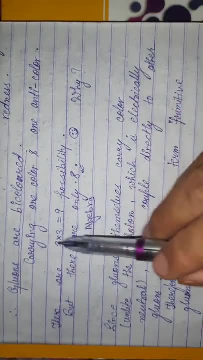 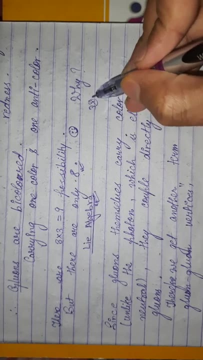 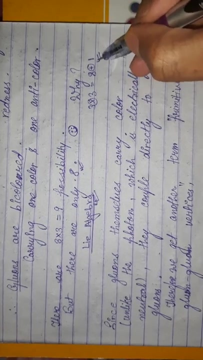 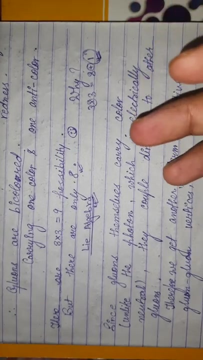 find i mean color combination that we can found. okay, because of the lee algebra. when you go to lee algebra, you will find that three cross three, in case of lee algebra converts into eight plus one, and this one is of something contradiction. and this one actually contains three, uh, three color and anti-color pairs. okay, this one contains three color and. 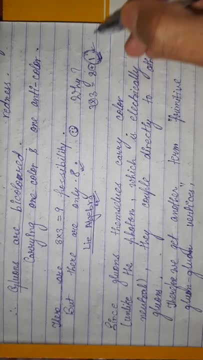 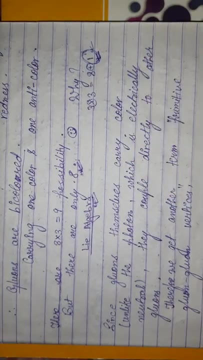 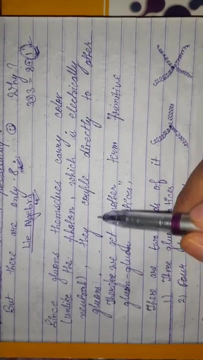 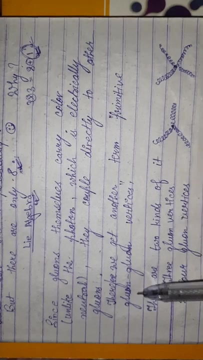 anti-color pairs. so we disregard it for now and we will look at only eight. eight of the gluons. okay, moving forward, since gluons themselves carry color, unlike the photon, which is electrically neutral, they couple directly to other gluons. okay, this one is important. therefore we get another term: primitive gluon, gluon vertices. earlier we had we had that. 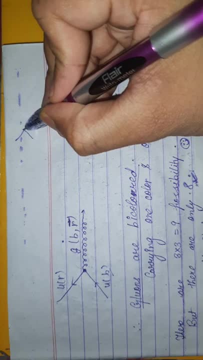 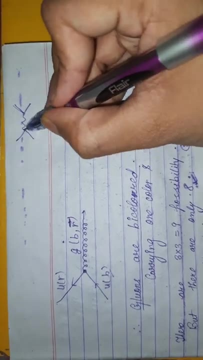 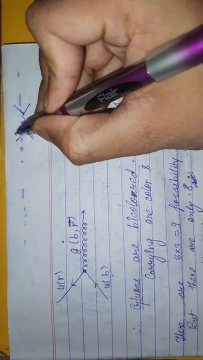 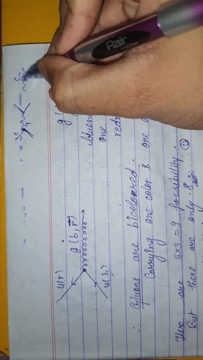 when two electrons are approaching each other, we have a photon and then we have another two electron moving away from each other. now we saw here that there is a vertices that involves both photon and electron. there is no vertices like this: photon and then photon, and then photon and then photon. this in this one cannot be called vertices, because 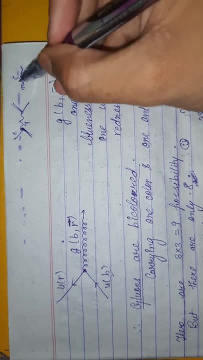 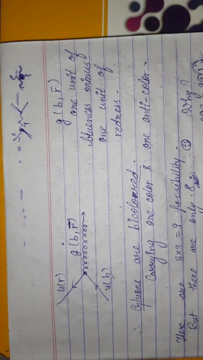 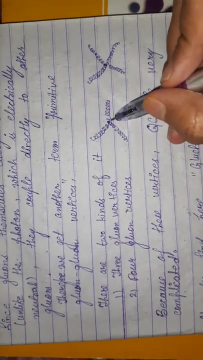 photon represent only uh, one, uh, only one particle- i mean one representation- and does not form vertices by combining in itself. but gluons can. gluons can combine with each other and form vertices, like this one and this one, because of the fact that gluons are made up of different. 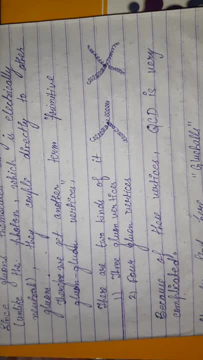 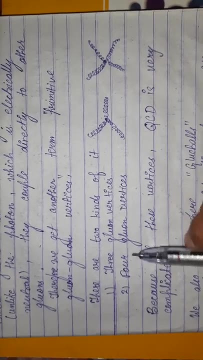 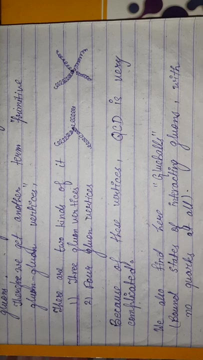 colors. okay, but photons are of similar type, so they don't form vertices. there are two kinds of it: three gluon vertices and four gluon vertices. okay, because of these vertices, qcd is very, very complicated and we will later know why. okay, we also find here glue balls, bound states of. 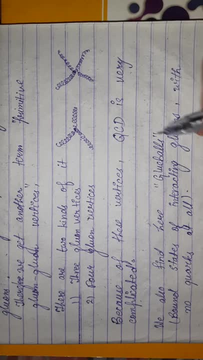 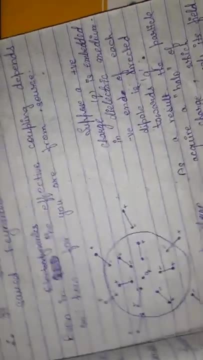 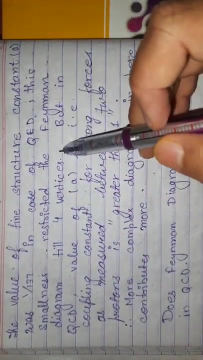 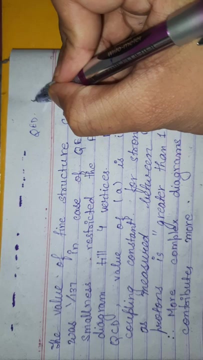 interacting gluons with no quarks at all. it is also possibility that we will ponder upon glue balls. glue balls contains only only gluons but no quarks at all. okay, the value of fine structure constant in case of qed. in case of qed, the value of fine structure constant was 1 by 137, but in case of qcd, the value of fine 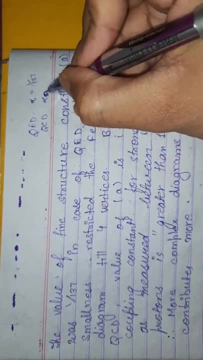 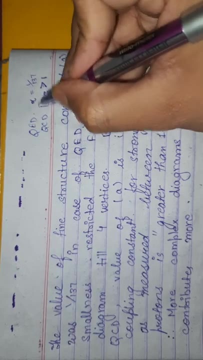 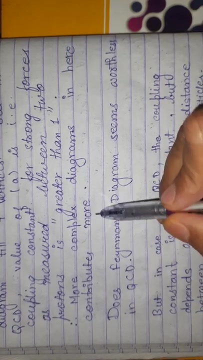 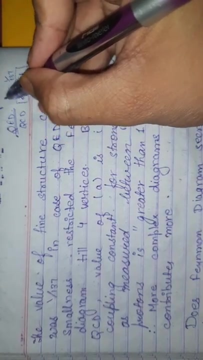 structure constant. or you can say coupling constant. you can say coupling constant is something around, is something more than one, something more than one. okay, more complex diagram in here, completes, contributes more. we have seen that in qed after four, after four vertices, we don't after four vertices, we don't care about the diagrams. 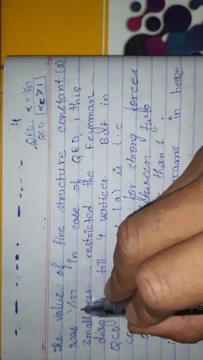 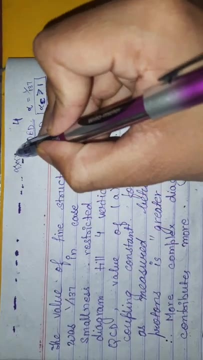 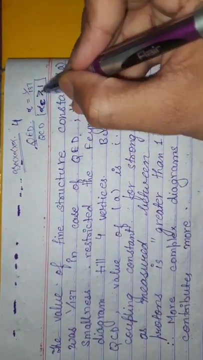 but in case because of the fact that the coupling constant, i mean the fine structure constant- was very small and when it is further multiplied it gives more small value, which is of negligible influence. but if the value of coupling constant is greater than one, that means the more the diagrams 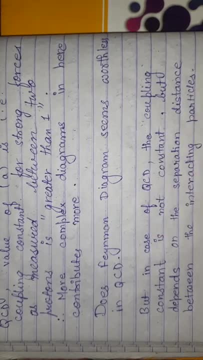 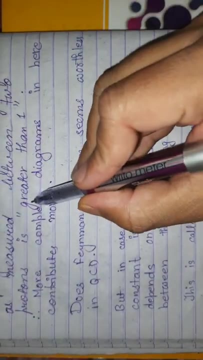 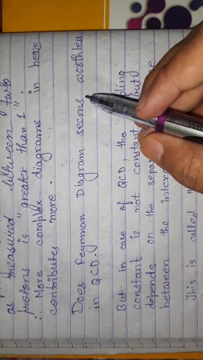 contribute. okay, so it is a bit of a confusing term now. does find my diagram seems worthless in qcd after coming to this fact that constant, that alpha, is greater than one. we could say that find my diagram is worthless in case of chromodynamics, but in case of quantum chromodynamics, 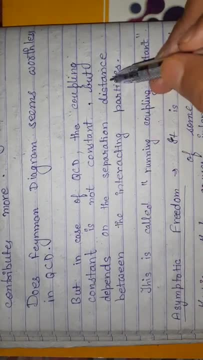 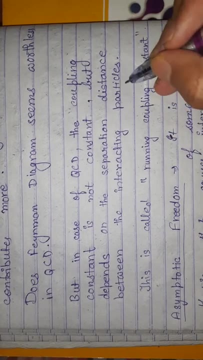 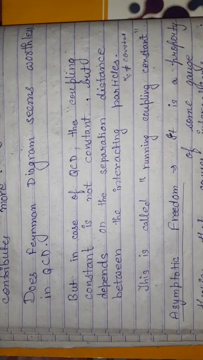 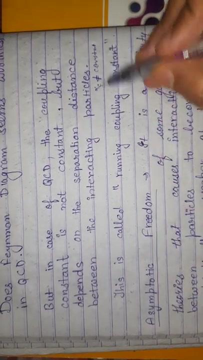 the coupling constant is not constant but depend on the separation distance between the interactors, the interacting particle. okay, this one is very important. here we should know that the coupling constant is not constant. it is not constant, but it is variable and it depends on the separation between the interacting particles. okay, this, these types of couple constants are called. 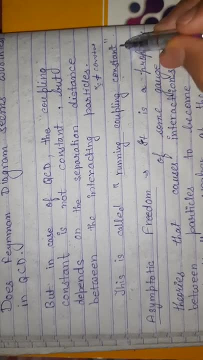 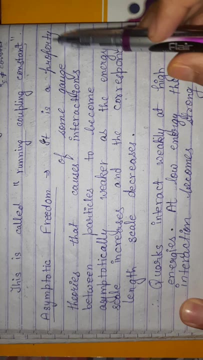 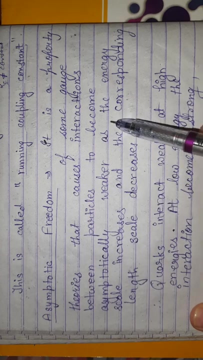 i mean coupling constants are called running coupling constants. okay, now, this is a very important term: asymptotic freedom. it is a property of some gauge theory that causes interactions between particles to become asymptotically weaker as the energy scale increases and the corresponding length scale decreases. this is very important, you should know. 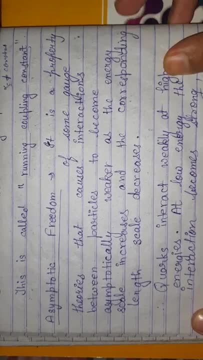 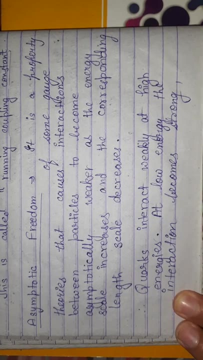 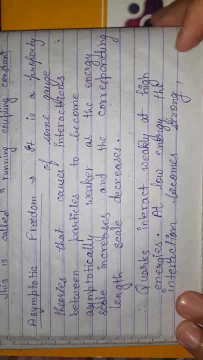 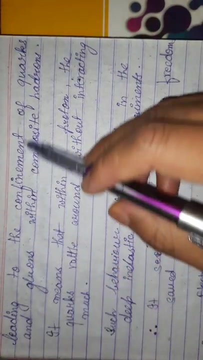 but after reading these terms you might get confused, so i will directly go to the. some properties, like quarks, interact weakly. at high energy that means the more the energy is, the interaction is less okay. at low energy, the interaction becomes strong. that means the low the energy, the more interaction it get. this leads to the confinement of quark. 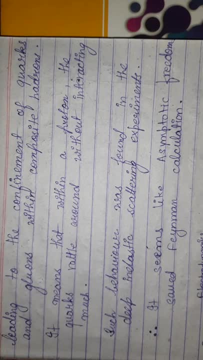 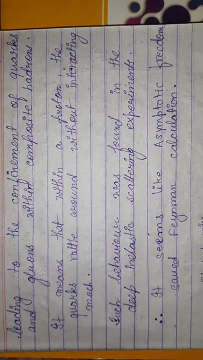 and gluons within compose, within composite hadrons. we know that hadrons are made up of quarks and gluons, so actually that property binds to quarks and gluons with each other to form hadrons. okay, it means that within a proton the quarks rattle around. 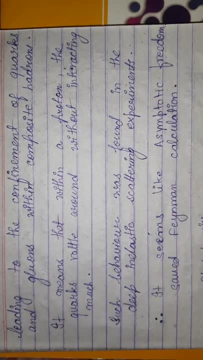 without interacting much. in in case of a proton we, if we consider a proton, the length scale is very low and the energy scale is very high. in that case the interaction is very low, as we can see that when energy is high, the interaction is low, and when the energy is high, the interaction 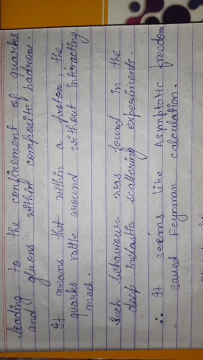 is low. another possibility is that whenKelly is very low, then the energy is very high. okay, so you can. this is also the same principle is there. so this is basically why in Adobe, energy is low, interaction is high. thus we can say that within a proton quarks can move. 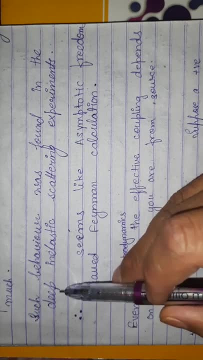 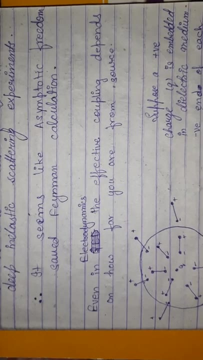 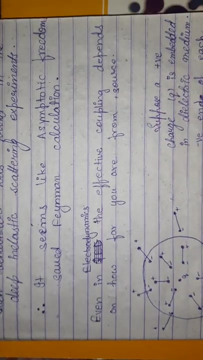 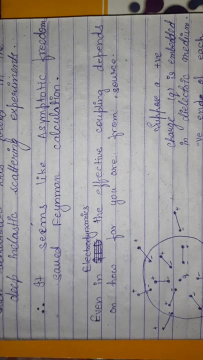 freely. such behavior was found in the deep elastic, inelastic scattering experiments that we will go later on. it is a very deep topic, therefore. it seems like asymptotic freedom shapes Feynman calculus. obviously it saves the Feynman calculation in this way. asymptotic freedom is thus important, very important, and you should know it, even in electrodynamics. 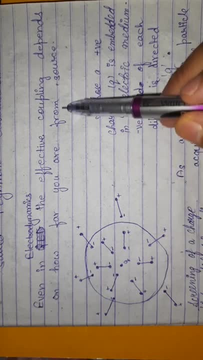 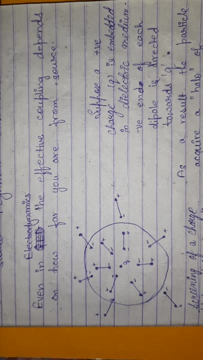 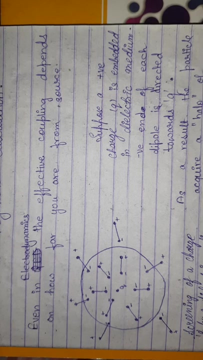 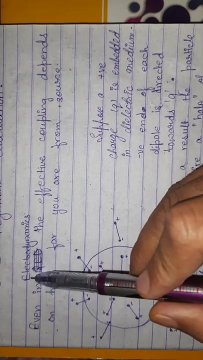 the effective coupling depends on how far you are from the source. it is not only applicable in quantum chromodynamics, that, as that, as far you go from one particle to another, the interaction become high. it is not only applicable to quantum chromodynamics, but also applicable in normal electrodynamics and in case of quantum electrodynamics. okay, let's see normal electrodynamics. 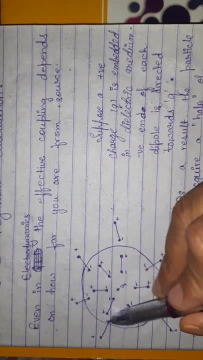 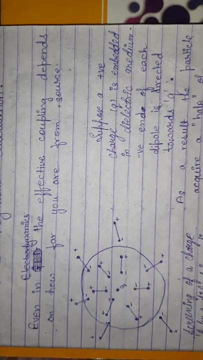 in case of normal electrodynamics, consider this as a. consider this as a dielectric medium where we have placed a charge positive charge plus q. now, if this is a dielectric medium, it has molecules which can be polarized and those polarized molecules become positive because they are polarized and those polarized molecules become positive. 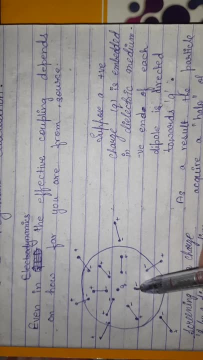 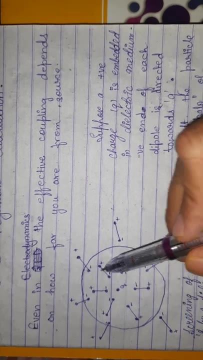 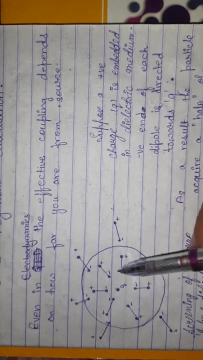 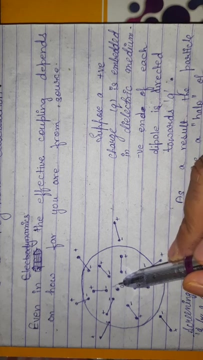 and those polarized molecules become directional. the negative, the negative part of the molecule gets attracted towards positive charge and the positive part of the molecule gets away from the plus q. okay, in this case it is arranged in this way. this is arranged as so we can say that the near, the more near we are to the charge, the more effect of charge we get. 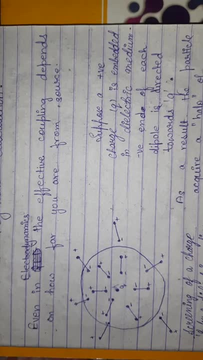 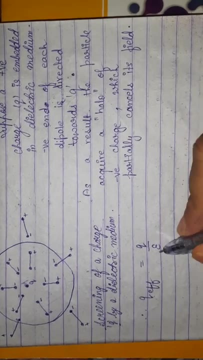 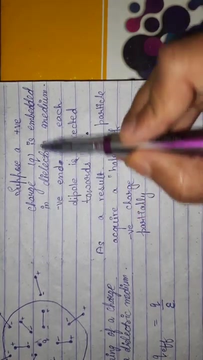 and the farther we are we get the less effect of this charge. so from there we get to the fact that q effective is equals to q by epsilon, where epsilon is the permittivity. okay, i can read it for you. suppose the positive charge is embedded in dielectric medium negative end of each dipole. 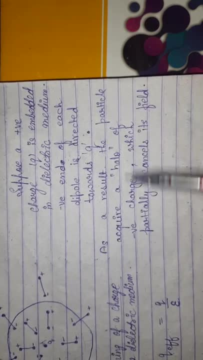 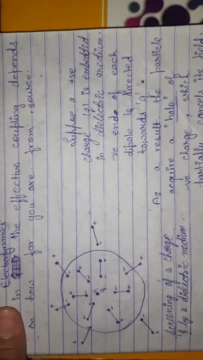 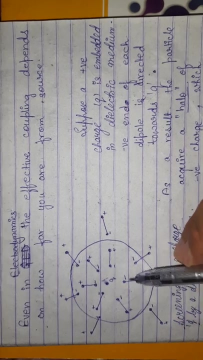 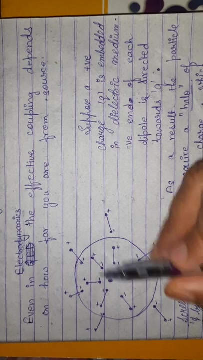 directed toward q as a result. the particle require i mean acquire a hollow hollow of negative charge which partially cancels its field. that means that these negative charge acquires a hollow up, creates a hollow hollow. you can say a hollow means that the amount of electric field that this positive q charge is throwing. 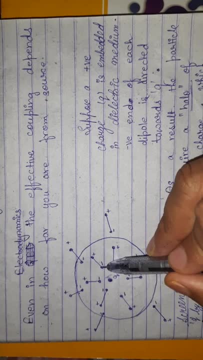 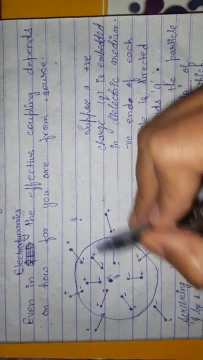 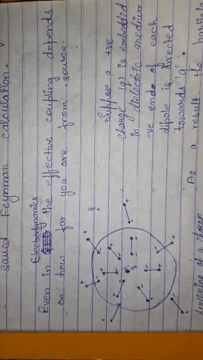 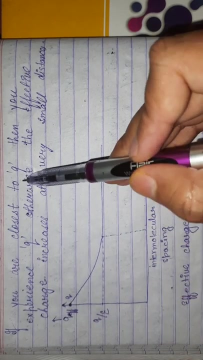 out of it is somewhat absorbed by these negative charge and the effect that a person is standing here or a charge here will be affected by this is very low and the electric field will that will that will approach here will be low. now if you are closest to q, then you experience. 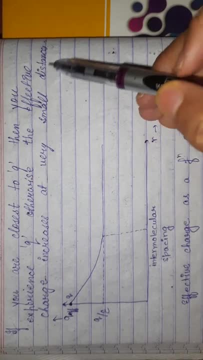 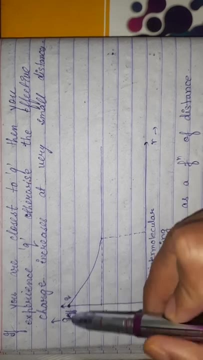 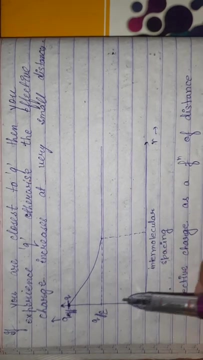 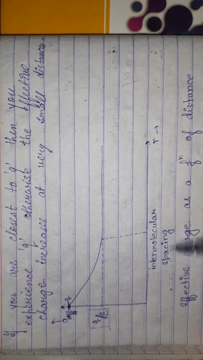 q, otherwise the effective charge increases at the small, at very small distances. now here is a graph for q effective, and at the peak you can say: here is the original charge q, and then there is dielectric charge. q by e i mean the charge that is influenced by dielectric medium, q by e, and it is a intermolecular spacing. 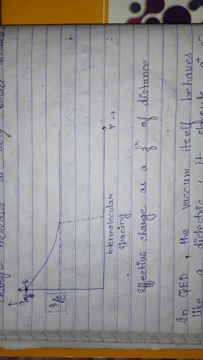 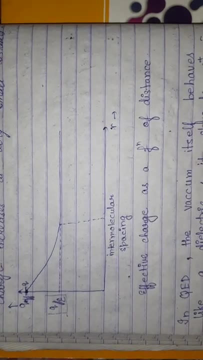 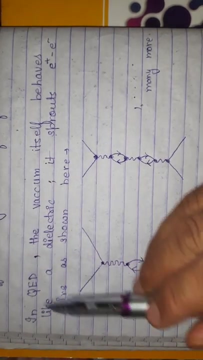 effective charge is a function of distance. this is the graph of effective charge is a function of distance. you can see that the charge is varying here with respect to distance, and it is similar with the quantum chromodynamics case too, now in case of quantum electrodynamics. 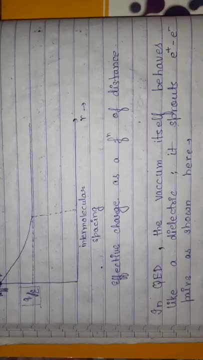 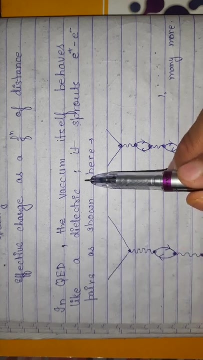 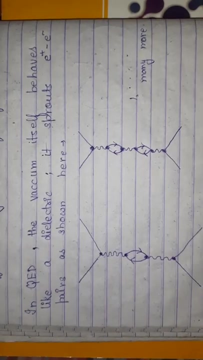 the thing that we learned here is that is only applicable to classical electrodynamics. now, in case of quantum electrodynamics, the vacuum itself behaves like a dielectric. it sprouts positron and electron pairs, as shown in the figure. in case of quantum electrodynamics, the vacuum vacuum present behaves like a dielectric. 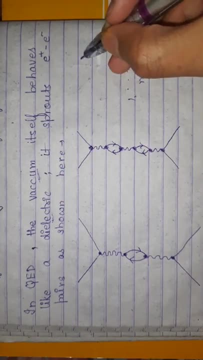 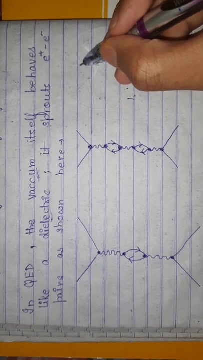 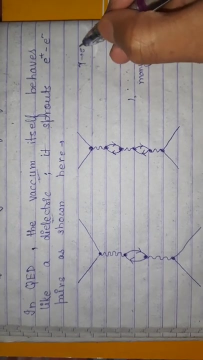 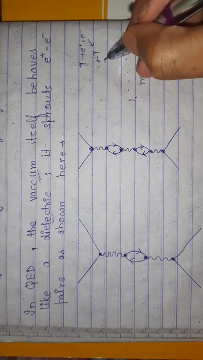 medium, because in vacuum we can say that there is nothing. and when then there, when there is nothing, we can assume that suppose there is some photon traveling around and that photon could easily be converted into a positron and electron. then this positron and electron annihilates into photon, then further it dissociates into- i mean pair production, into electron. 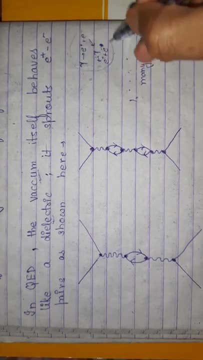 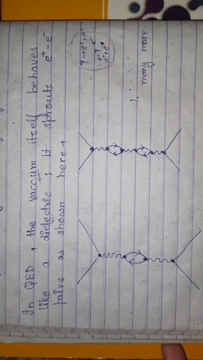 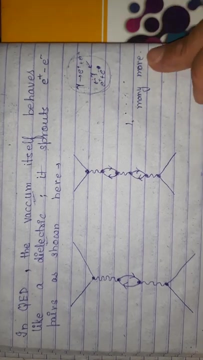 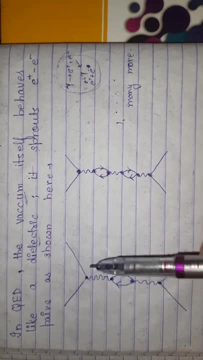 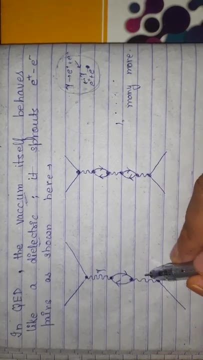 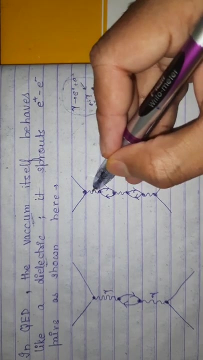 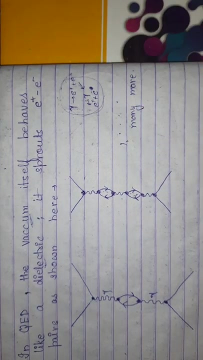 diagrams in which you can say that two electrons are coming here, but they get influenced by photon, then photon dissociates into electrons, then for then they all produce photon and then they dissociate into electrons. similar thing goes here and it and the number of loops that here we can see can increase to infinity. 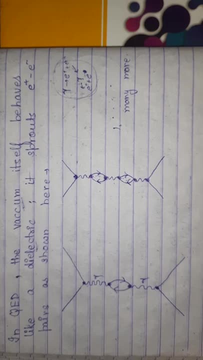 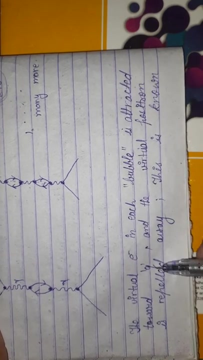 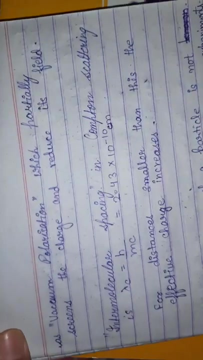 okay, now how does this become a dielectric medium? that is of importance. the virtual electron in each bubble is attracted towards positive charge q and the virtual positron is repelled away. this is known as. this is known as vacuum polarization- very important vacuum polarization. 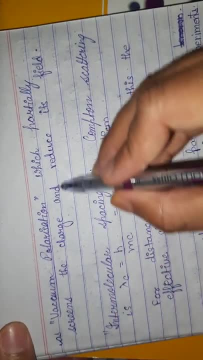 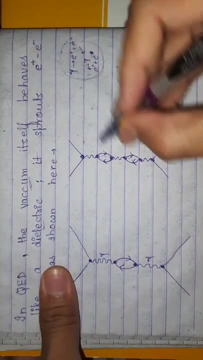 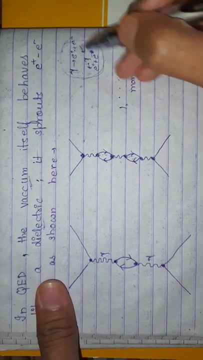 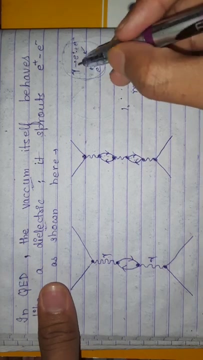 which partially repels the vacuum, so actually screens the charge and reduce its field. that means, let me tell you this very clearly: suppose there is a photon out of nowhere. there is a photon and it creates a electron and positron whole pair. okay now, since there is a proton somewhere in vacuum, and for the 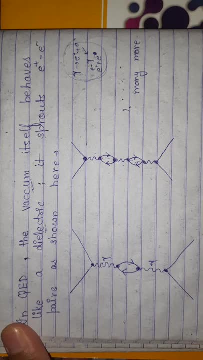 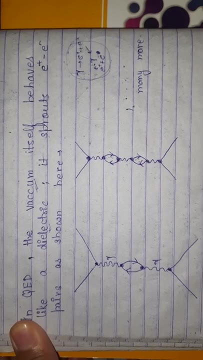 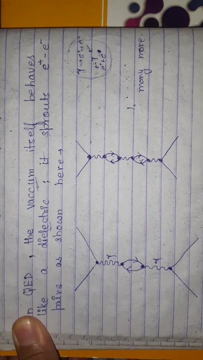 instant, when positron and electron are are formed, what will the proton will do? the proton will obviously try to attract the positron. I mean attract the electron and repel the positron and for that moment there will be a dipolar, a dipolar. 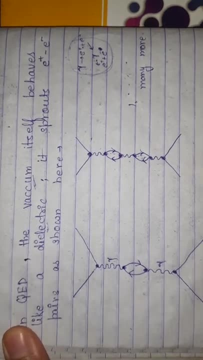 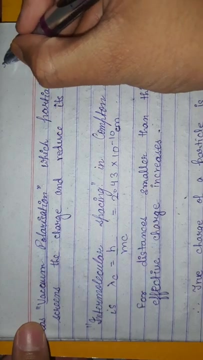 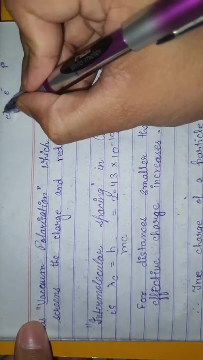 I mean there will be a situation of polarity. there will be a situation of polarity and in that case of, and in that situation of polarity, when there is suppose there is a proton which at is attracting electron and repelling positron, then some of the electric field gets used. 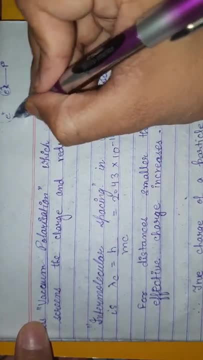 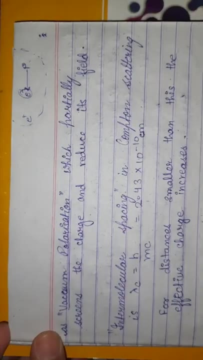 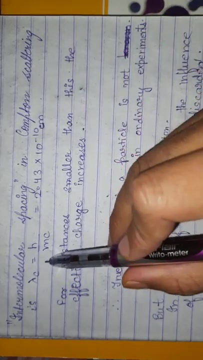 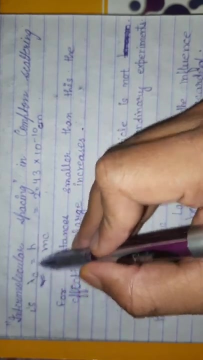 by this electron and the actual effect that we get from our laboratory gets reduced. okay, this is very important. now, intermolecular spacing in Compton scattering is this: this is also called a Compton wavelength, Compton wavelength, Compton wavelength- This is called Compton wavelength, where lambda c is h, y, m, c. m can be written as m, e, rest mass. 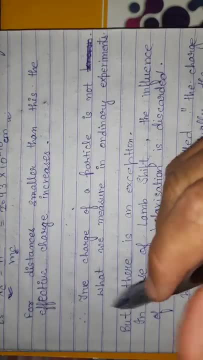 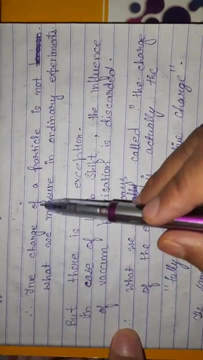 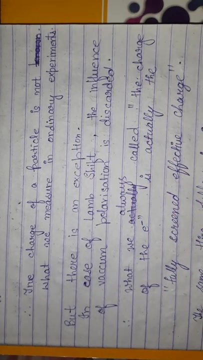 of electron and the value is something like this: for distances is smaller than this, the effective charge increases obviously. now, true charge of a particle is not what we measured in ordinary experiments. we have got the value of true charge as 1.6 into 10 to the power. 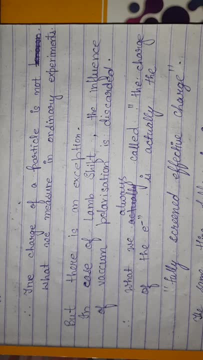 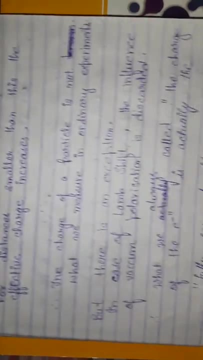 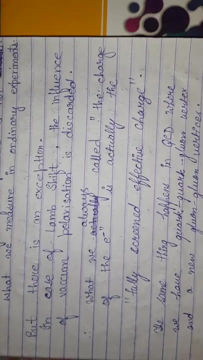 minus 19 or something, But. But that is actually not accurate. there is still some hindrance because of the vacuum polarization. okay now, but there is an exception. obviously there is an exception because we are in high energy physics, we are probing in further, we are going in, we are going into. 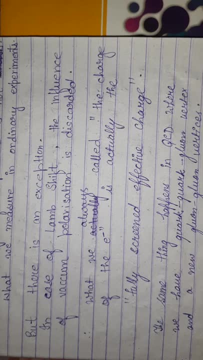 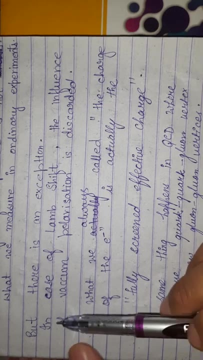 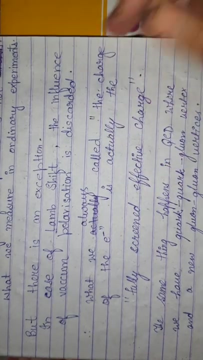 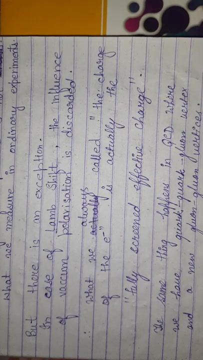 the minute levels. I mean, while we are, we do experiments with a spectrum, we go at very minute lengths. okay, So in case of lamp shift, lamp shift is basically responsible for hyperfine splitting. okay, so in case of lamp shift, the influence of vacuum polarization is disregarded because the distance 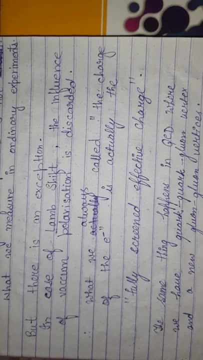 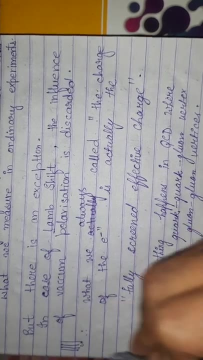 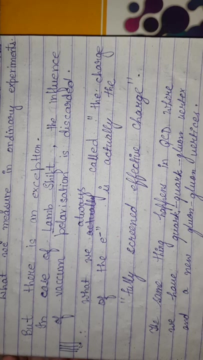 between two, two, you can say the distance between the spectrograph that we get in case of lamp spectra, So, So, So it's too small and we can say that there is not enough space for an electron and positron to be created and thus, in case of lamp shift, sift, the influence of 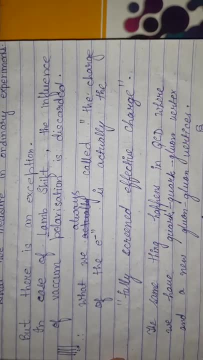 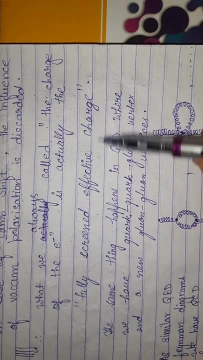 vacuum polarization is disregarded or discarded. okay, What we always called the charge of electron is actually the fully screened effective charge. now, this is a very important term. What we called the charge of electron is actually the fully screened effective charge. now, this is very important term. 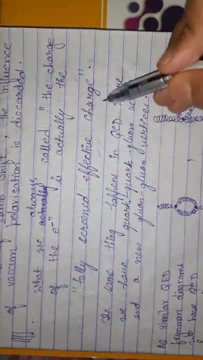 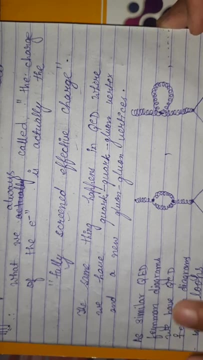 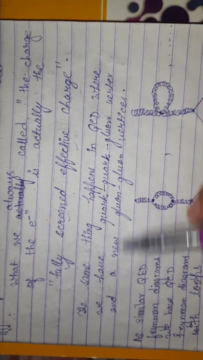 Now this is very important term, actually- the fully screened effective charge, because it is getting screened by vacuum, also because of the electron and hole pair. The same thing happens in quantum chromodynamics, where we have quark, quark gluon vertex and a new gluon gluon vertex, As I told earlier that we have. 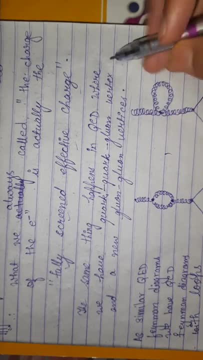 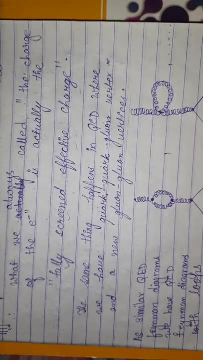 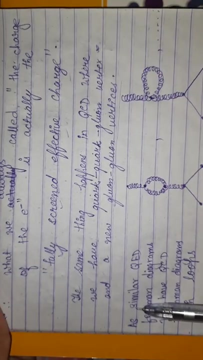 a new vertex here, gluon gluon vertex, and this one is very familiar to you. You can also call it as electron electron photon vertex or, in case of QCD, quark quark gluon vertex. Now, as similar to quantum electrodynamics Feynman diagram- we have quantum chromodynamics. 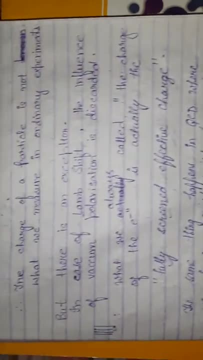 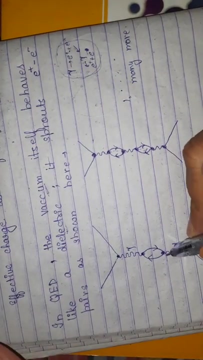 Feynman diagram with loops, The loops that we created in case of quantum electrodynamics, here that there will be some positron and electron which could hinder the actual electron from the quantum chromodynamics. So we have quantum chromodynamics with loops. 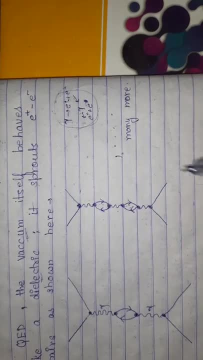 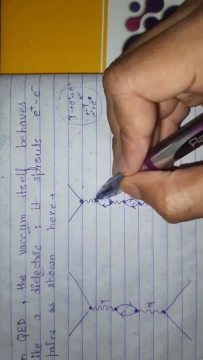 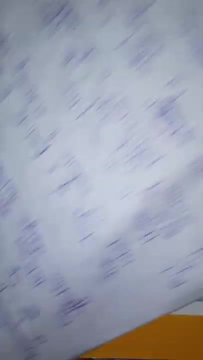 They are there at the end of the quark quark vertex. So we can also say that the electron growth is strong enough to let the electron move in time and to charge off a particle. Now, here, in case of a gluons, and in case of gluons and quarks, we just replace these lines. 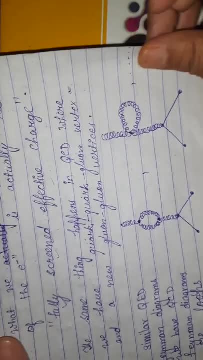 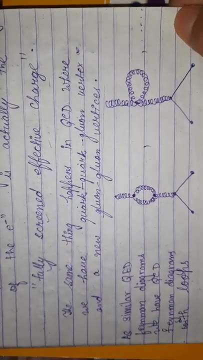 and we get them and we, we get the same amount of vacuum in here. I mean, I mean we get the same empty space and here also some hindrance happens and the actual effect of gluon and quarks are not constant, not available. they get some hindrance by vacuum too. ok, 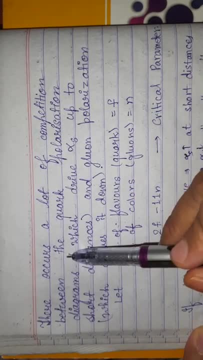 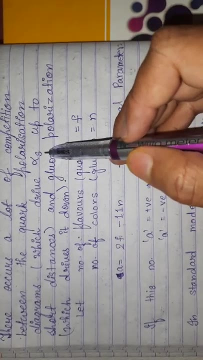 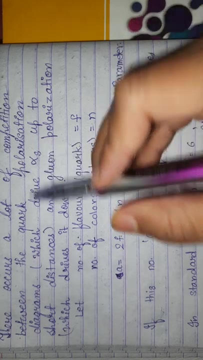 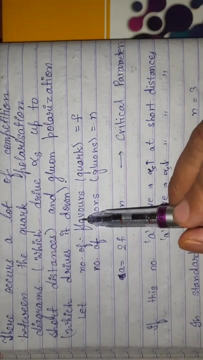 Now there occurs a lot of competition between the quark polarization diagrams, ok, which drive alpha s. alpha s, as I told you earlier, it is actually the, it is actually the critical constant which drive alpha s up to short distances, and gluon polarization which drives it down. 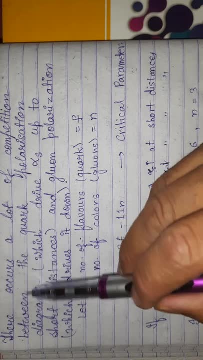 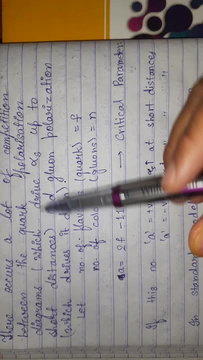 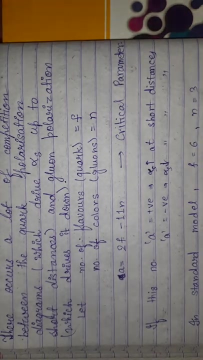 ok, now this is very important to know that there occurs a lot of competition between quark polarization. I mean polarization could be of many types. polarization could be done by quark or could be done by gluon. now, which one effect more that is important in case. 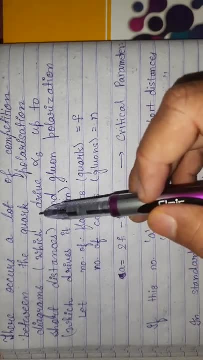 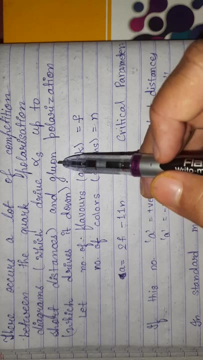 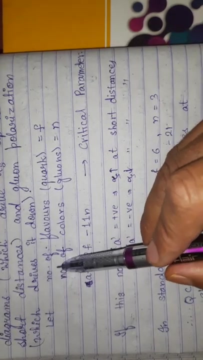 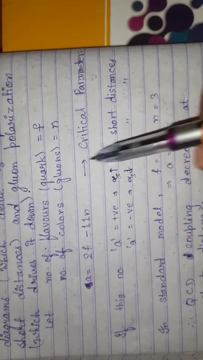 of: if quark is Having some polarization, then the constant the constant is increased, and if the gluon is having polarization, then the constant is decreased. ok, now consider these variables: number of flavors, number of quarks is equals to f and number of color gluons is equals. 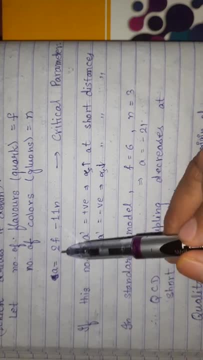 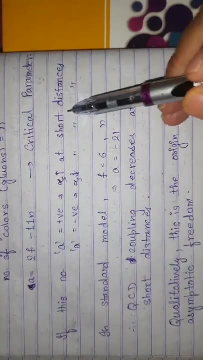 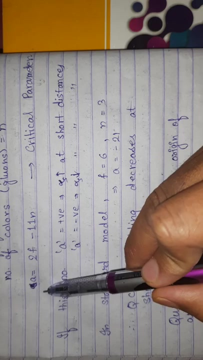 to n. here is the formula: a is equals to 2f minus 11n. it is also called as critical parameter. if This number is positive, then critical constant increases at short distances, and if this value is negative, then critical constant decreases at short distances. ok, 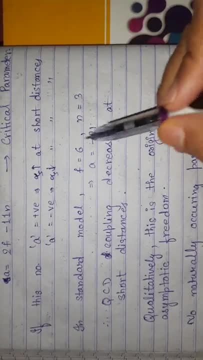 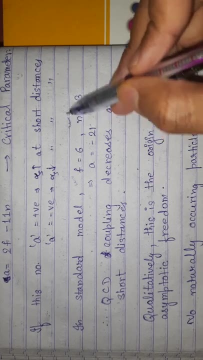 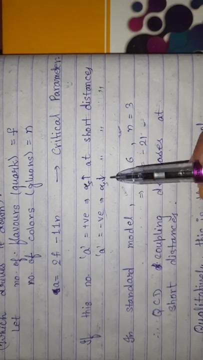 In case of a standard model where we know that the number of flavors- I mean the number of quarks- are 6 and the number of colors that we know are 3, there the value is a is equals to minus 21.. So the a is negative. that means that critical constant decreases at short distances. 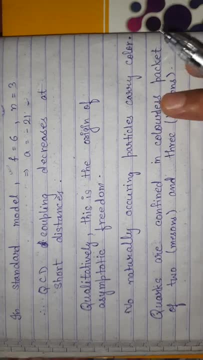 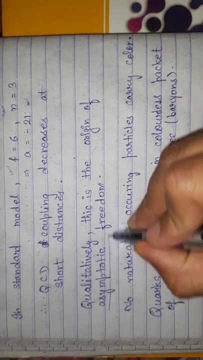 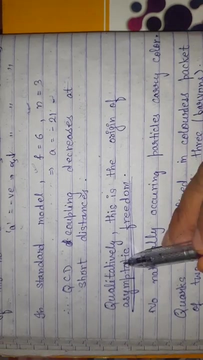 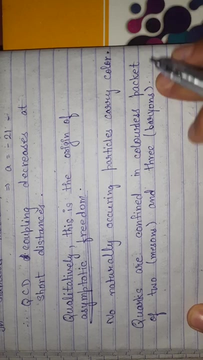 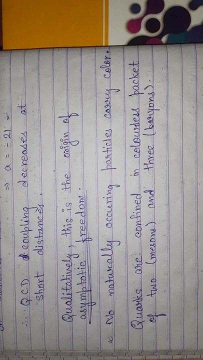 Now quantum chromodynamics: coupling decreases at short, short distances. this one is very important. ok, now qualitatively. this is the origin of asymptotic freedom. the thing that we learned earlier about asymptotic freedom is qualitatively- I mean qualitatively- proved here. This is a very important thing- that when we are saying that a particle is not the natural, 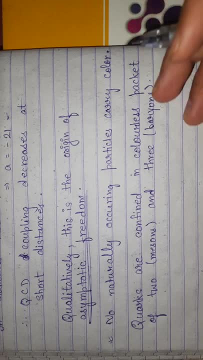 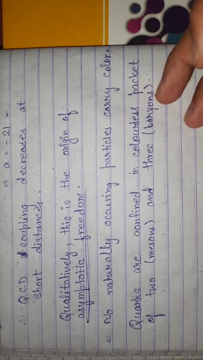 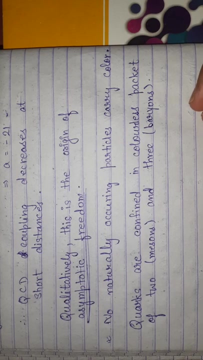 state, but that a particle is a natural state. there is no natural structure in which any particle has any color, So no naturally occurring particles carry color. this one is very important: that there is not a single particle that carries color, Because So quarks are confined in colorless packets of two and three. 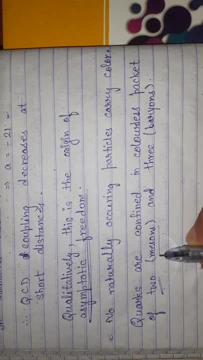 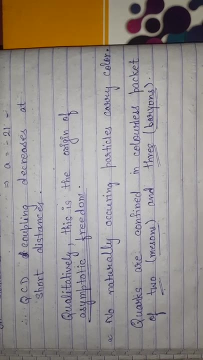 If there are two quarks which are confined, then it is known as mesons. If there are three quarks that are confined, then they are baryons. But this is to be embedded in your head that all these mesons and baryons are colorless. 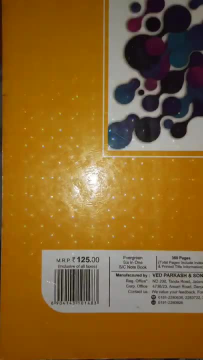 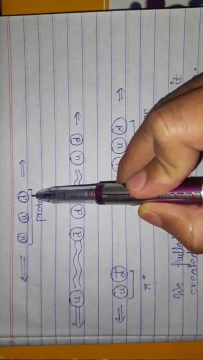 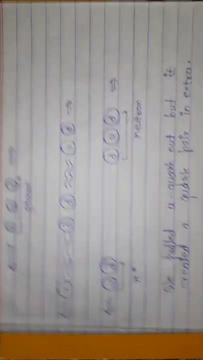 All of them are colorless. Okay, Now moving on. Suppose we have a proton and proton consists of up, up and down quark. Now we want to separate an up quark from this. We are pulling the up quark with all our might. 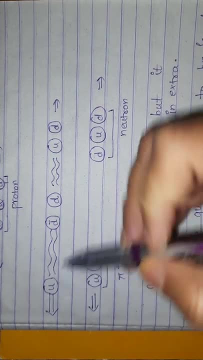 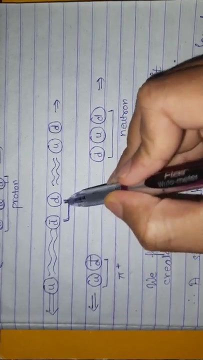 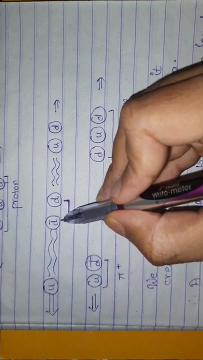 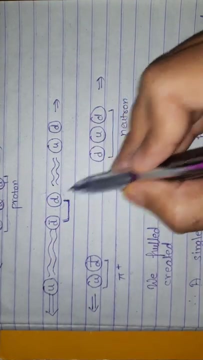 Okay, Now when we are pulling an up quark, there is a formation of down and anti-down quark inside the vacuum. Okay, And there is U and D quark which are together. Now anti-D quark will form a baryon with U quark and this D quark will form neutron with U and D quark. 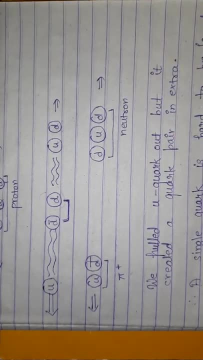 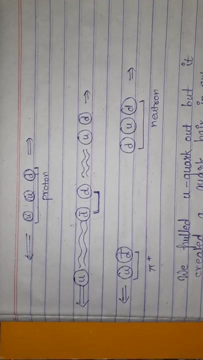 Okay, So what does this mean, actually, And what is the significance of this? quark and anti-quark is Now, as you can see, that this is actually a process that is very common, where proton is changed into neutron via baryon. So what does this mean? actually, We are pulling an up quark with U and D quark, and this is a process that is very common, where proton is changed into neutron via baryon. Now what does this mean? actually, You have learned it. 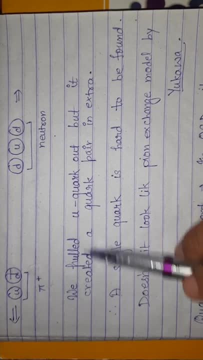 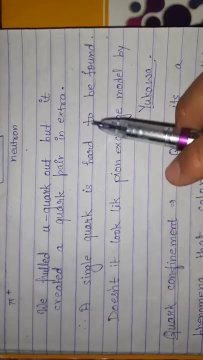 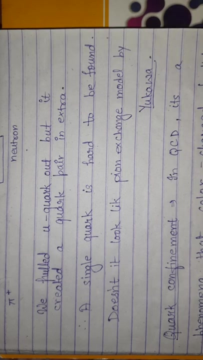 I mean, you have seen it or heard it somewhere. We pulled U quark out, but it created a quark pair in extra. A single quark is hard to be found. It is kind of not found. Okay, Doesn't it look like baryon exchange model by Yukawa? 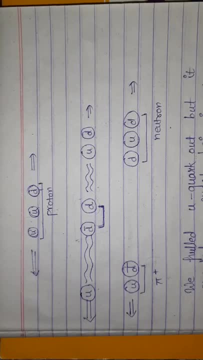 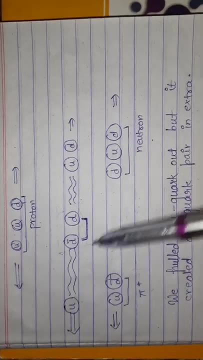 Okay, Now you remember that Yukawa baryon exchange model, is this model Very important model And you should know it. You should know this: How does this happen? Now, about this quark and anti-quark: we are going to discuss it right now.